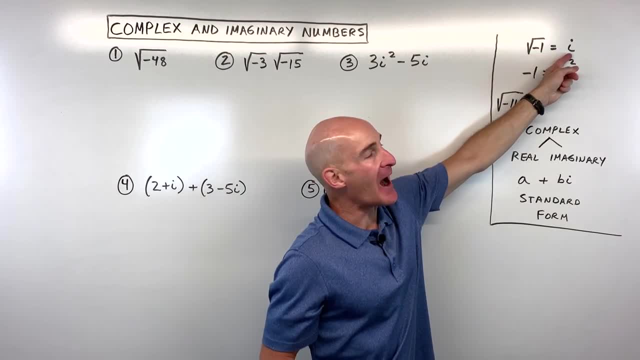 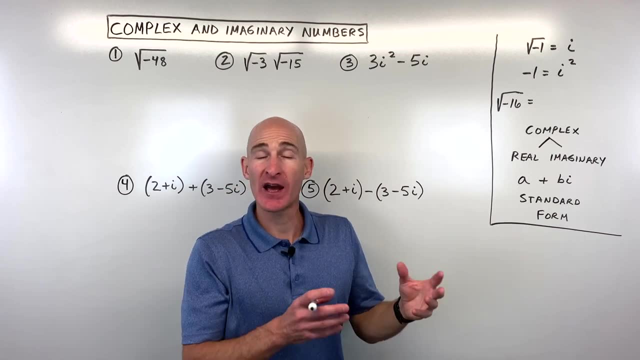 this right here: the square root of negative 1, we call that, i, for imaginary. Now we know, when you take the square root, like if I say what's the square root of 16,, we say what number times itself is 16, that's 4, right. But if we say what's the square root of negative 16,? 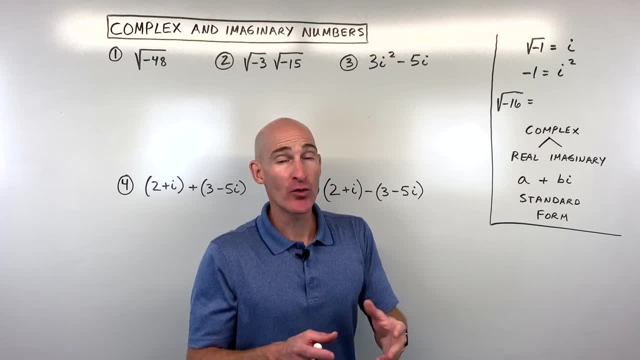 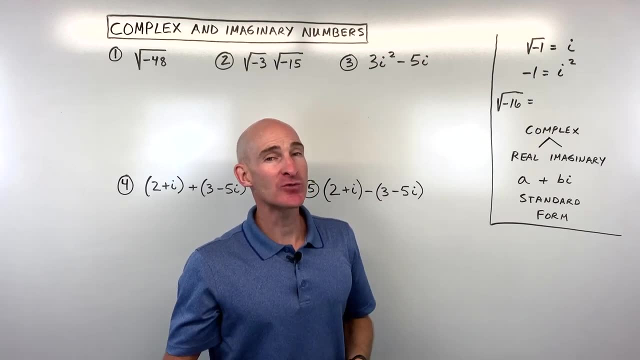 what would that be? Well, we can't say 4 times 4, that's positive 16, or negative, 4 times negative 4, that's positive 16.. So how do we take the square root of a negative number? That's where 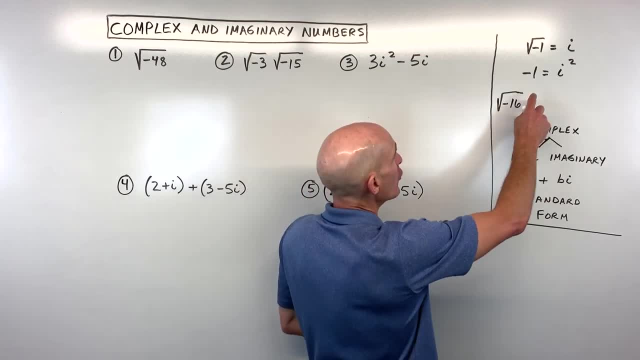 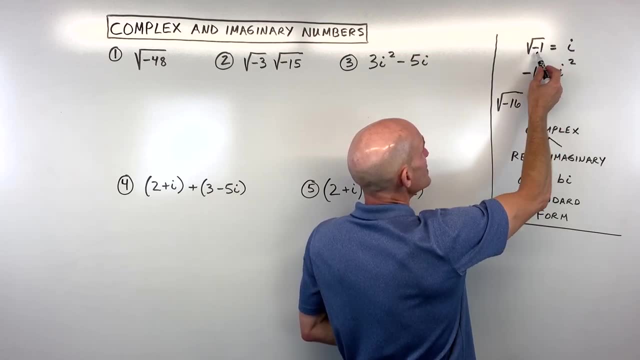 imaginary numbers come in Now. another thing you want to know about this notation here i is that if we square both sides of this equation, i squared is equal to negative 1. Because when I square the left side and the right side, the square and the square root cancel and 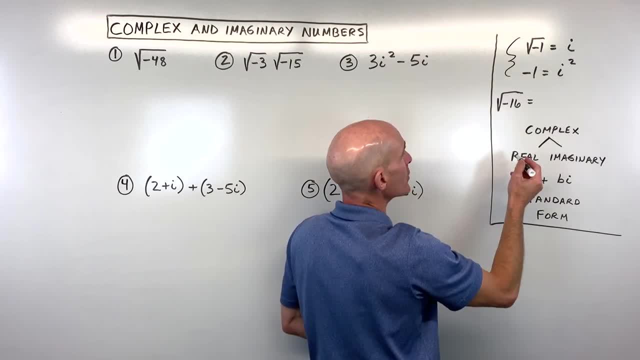 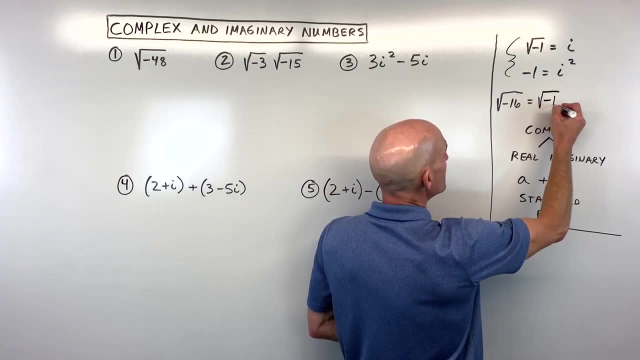 you're just getting negative 1.. So these are good to remember right here. But when I simplify a square root that's got a negative in it. what I like to do is split it up into two parts: Square root of negative 1 times square root of 16.. The square root of negative 1 is i, the square root. 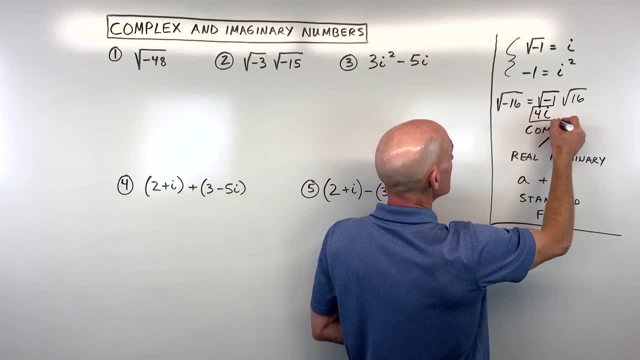 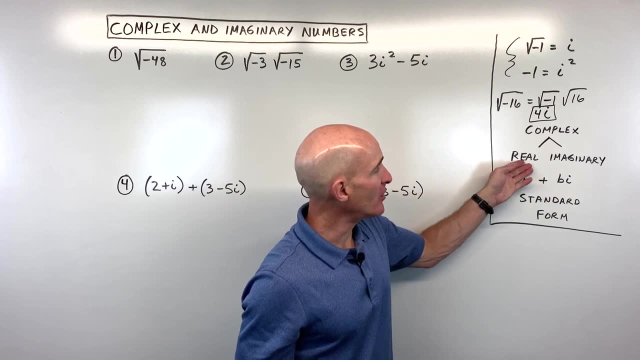 of 16 is 4, so altogether I would write this as 4i. Okay, now a complex number. what's a complex number? part real and it's part imaginary, And it's oftentimes written in this a plus bi form: The. 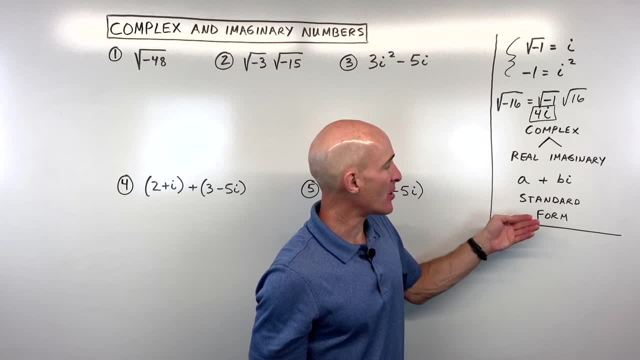 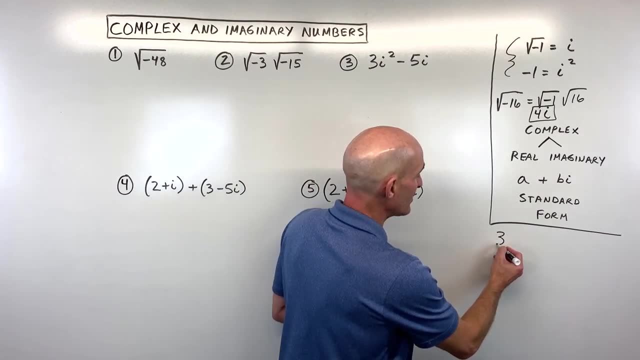 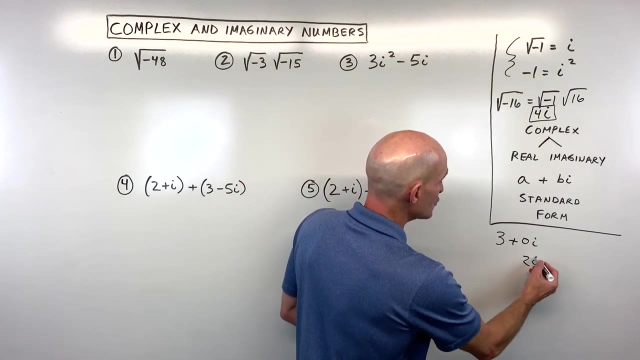 a represents the real part and the bi represents the imaginary part, And this is called the standard form of a complex number. So all these years, when your teacher was saying three, it was implied that it was three plus zero i, that there was no imaginary part. Or if you say, let's say two i. 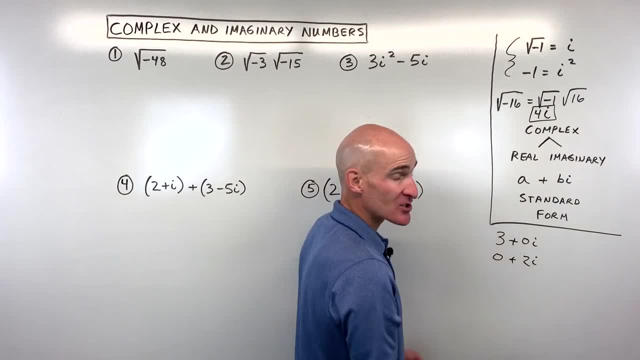 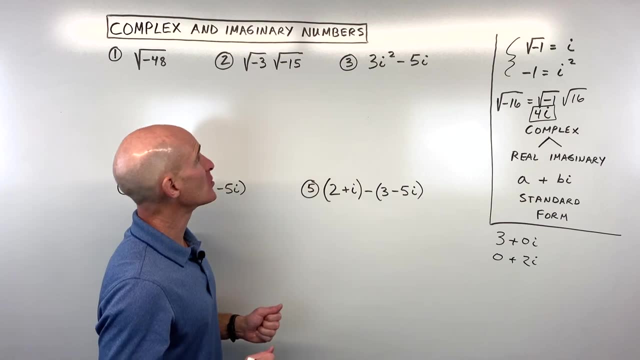 like this is imaginary number. it's really zero plus two i, But we don't oftentimes write the zero. But this is what a complex number is: part real, part imaginary. So let's get into some of these examples. This first one say we want to simplify the square root of negative 48.. 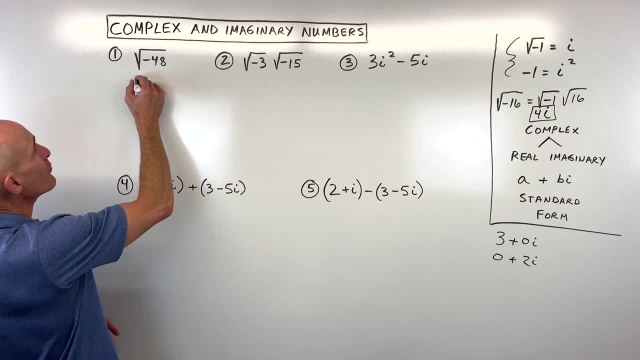 Well, what we can do is we can break this down. We could say: negative one times the square root of 48. So square root of negative one times square root of 48. That's the square root of negative one. we already talked about That's. 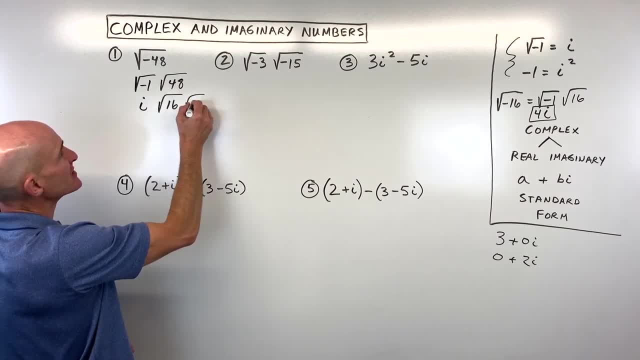 i 48,. we can simplify into square root of 16 times square root of three: That's 48.. And square root of 16 is a perfect square, That's four. So if we rewrite this now, we can write it as four i. 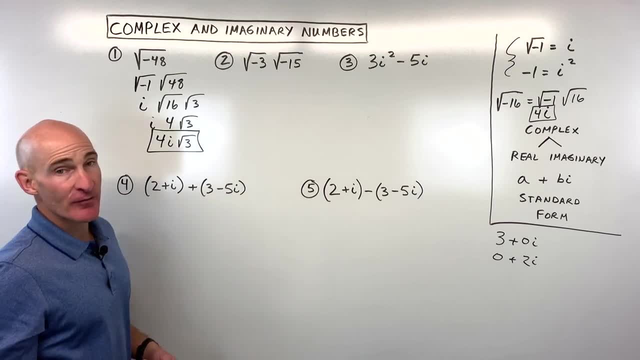 square root of three, And that's our final result. Now, sometimes students will mistakenly put the i over here, which you could do. The only thing is that it's oftentimes not written that way because it looks like the i might be underneath the radical. So to kind of avoid that, 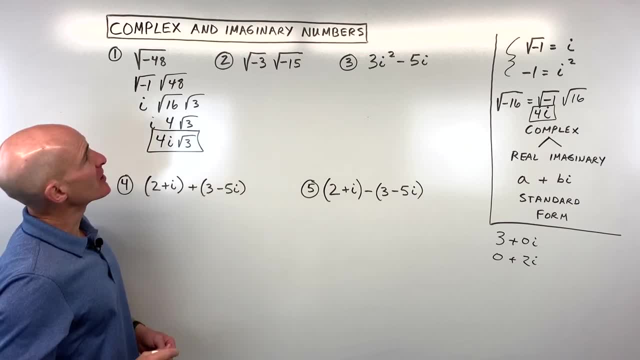 confusion, we're going to write it as four i square root of three, And that's our final result. So to kind of avoid that confusion, we usually put it up in front here. Let's look at number two now. So this one we have square root of negative three times square root of negative 15.. Now 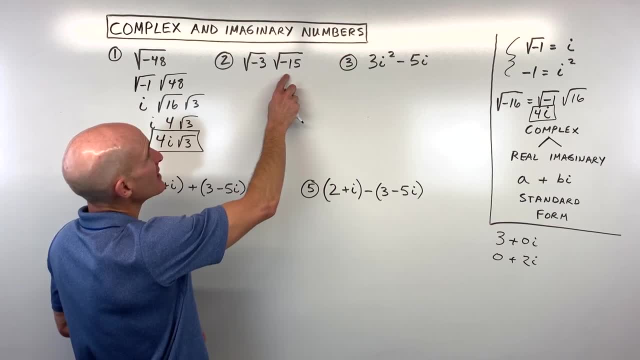 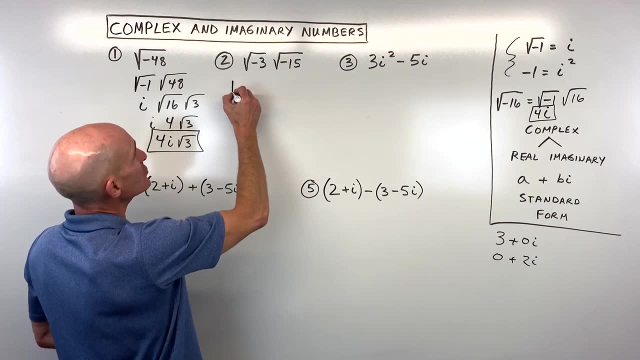 a mistake that students sometimes make is they just multiply these together and say, oh, that's the square root of 45, and simplify from there. You don't want to do that. What you want to do is you want to split this up into square root of negative, one times square root of. 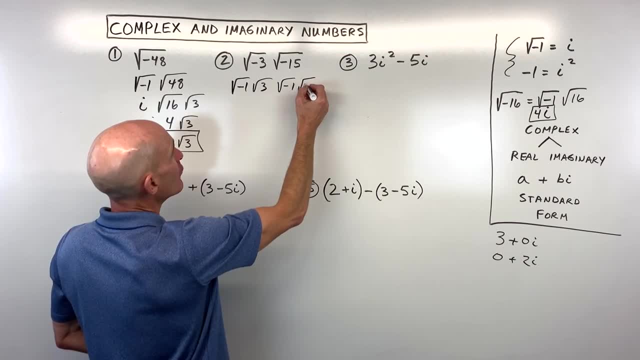 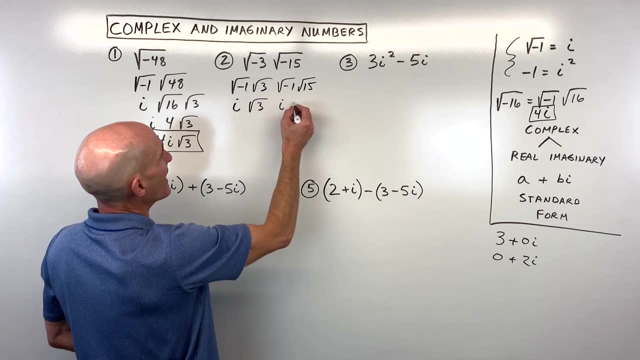 three, And square root of negative 15 is square root of negative one times square root of 15.. Square root of negative one we know is i, And this square root of negative one is i, And so i times i, we know is i squared Square root of. 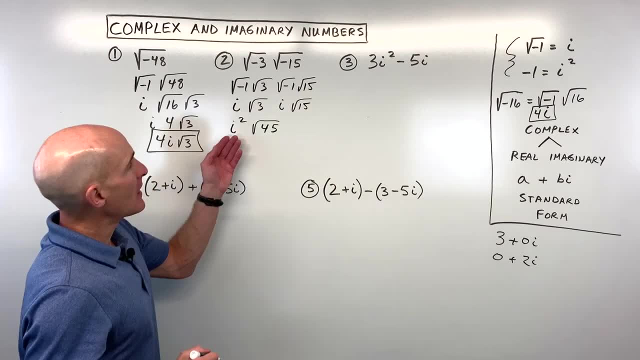 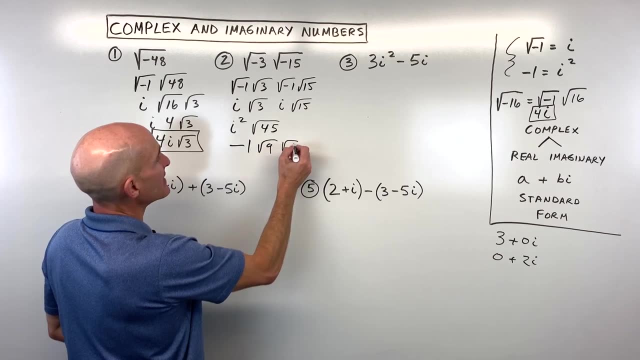 three times square root of 15 is square root of 45. And now we know i squared is equal to negative one And the square root of 45 is nine times five. Nine is a perfect square. That's three times negative one. This will give us negative three square root of five If we just multiply these together and 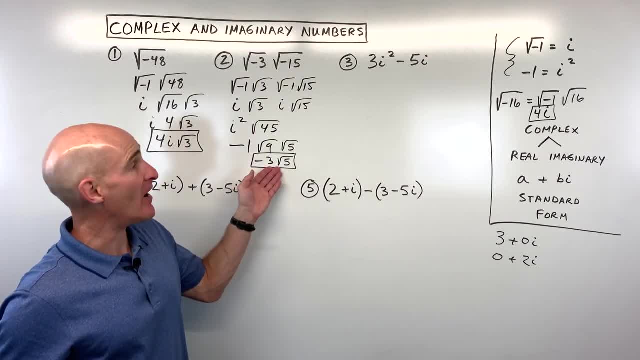 say square root of 45, you're going to get a square root of 45. And so i times i, we know, is i squared, We're going to get positive three root five. So you want to make sure you take that square root of. 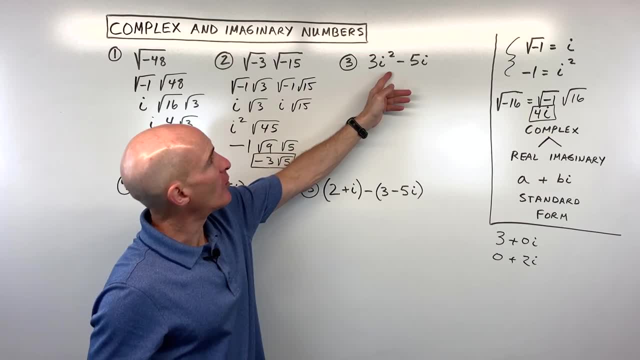 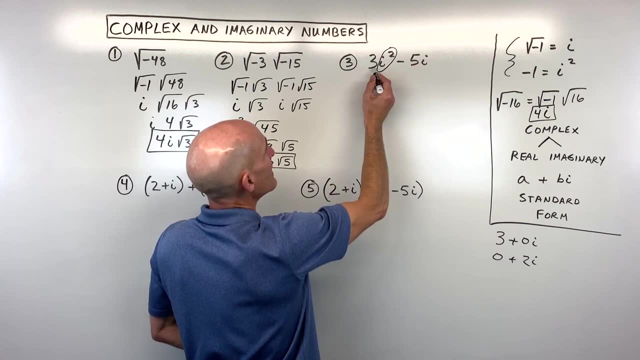 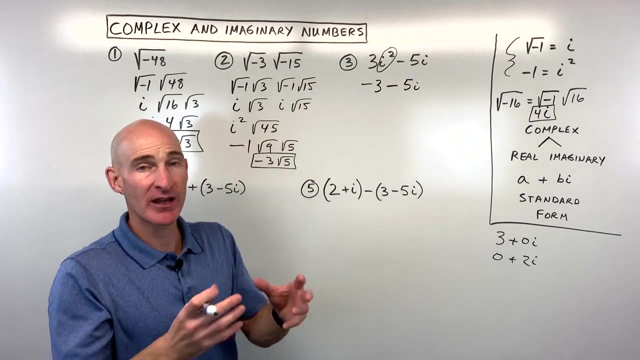 negative one out first. Okay, for number three. now, how do we simplify this one? Well, we can see, we've got that i squared in here. i squared is negative. one times three is going to give us a negative three minus five. i Now, we can't combine these because you've got an imaginary and a real. 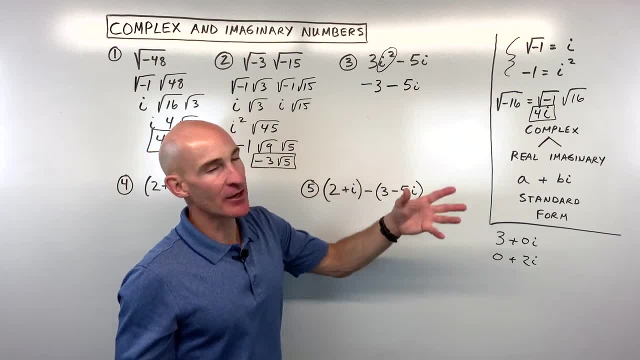 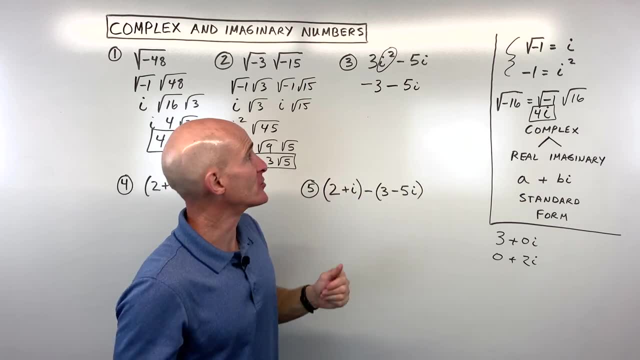 number and they're two different types of terms. You can kind of think of i as like a variable, like x or y or z, So you really can't combine them. You can't combine a number with a variable if you're just adding or subtracting. They're unlike terms. 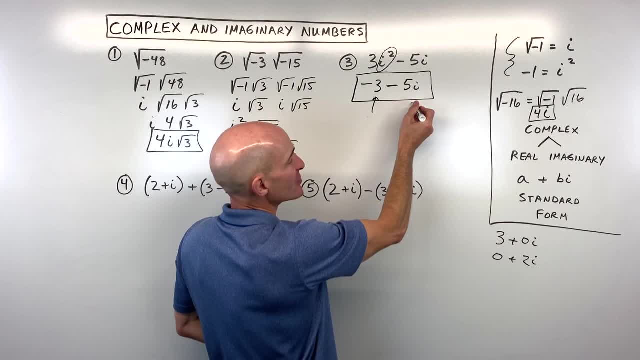 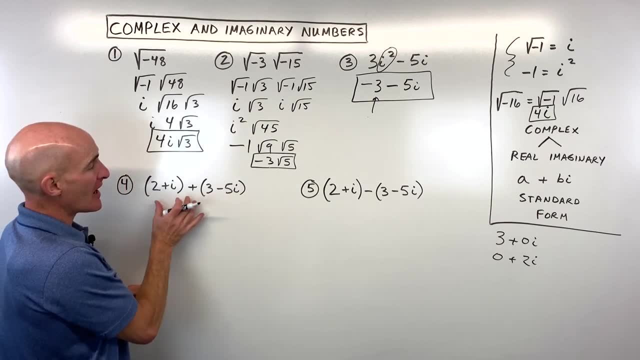 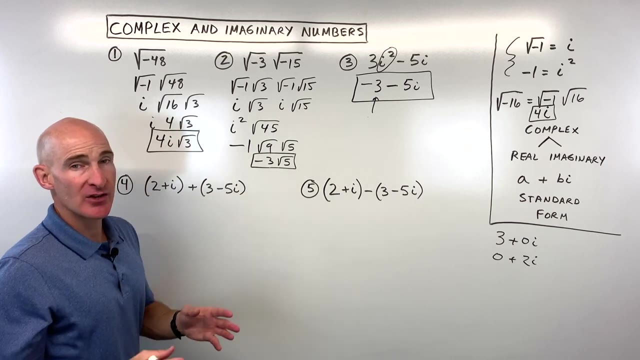 You also want to make sure you put this real part first and the imaginary part second in this a plus bi standard form. Okay for number four. now we're adding two complex numbers together. So again, just like we said, i can be sort of thought of like as, like a variable like x or y, And you can think 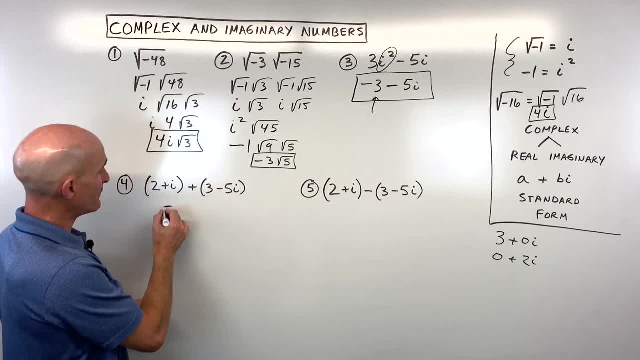 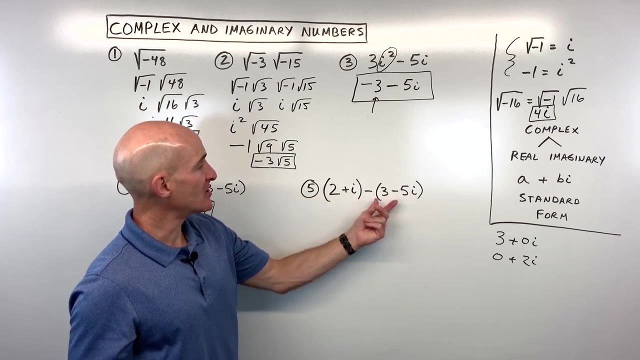 about just combining like terms. So we could say: two plus three is equal to five One i plus negative five i is negative four i. And that's in our standard form of a complex number, Real plus imaginary or a plus bi form Number five. we've got the same two complex numbers, but we're subtracting this time. 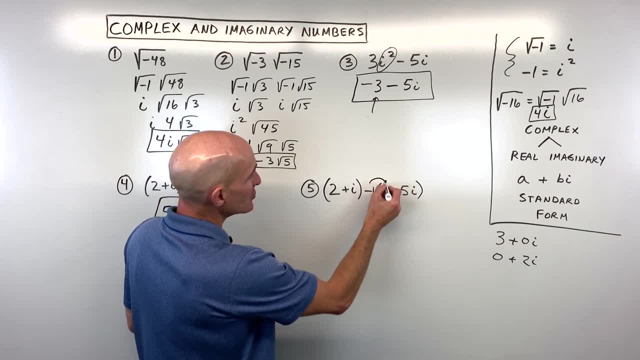 What you can do is you can think of this as like a negative one and distribute that negative one into the parentheses. So this is like negative three plus five i. And now all we have to do is combine like terms: Two plus negative three is negative one. One i plus five i is six i. 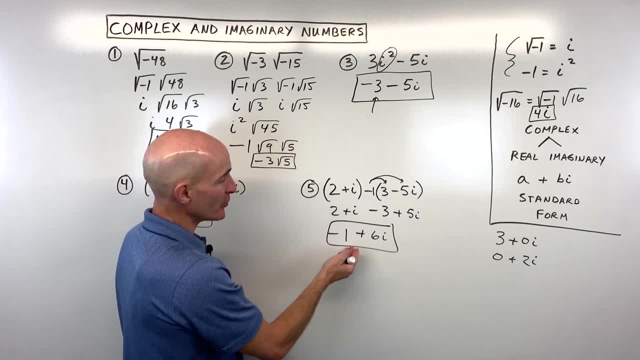 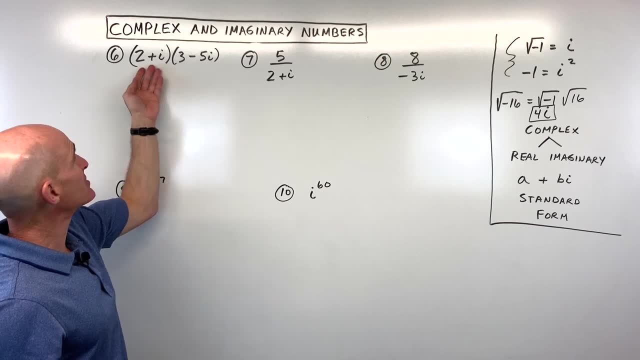 And we have it in these standard forms. Let's take a look at a few more examples. Okay, for number six. now we're multiplying two complex numbers together. You can see they're side by side with nothing in between. So multiplication. 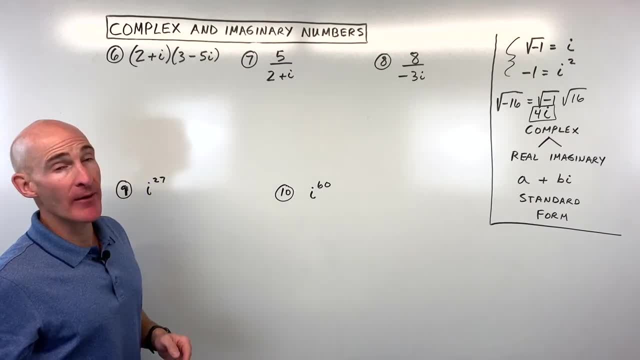 And here again you can think of that i as like a variable, like x or y, And so we have like a binomial times a binomial. We can do the FOIL method or the box method or the distributive property twice. Here I'll just distribute twice, I'll do two times three, which is six. 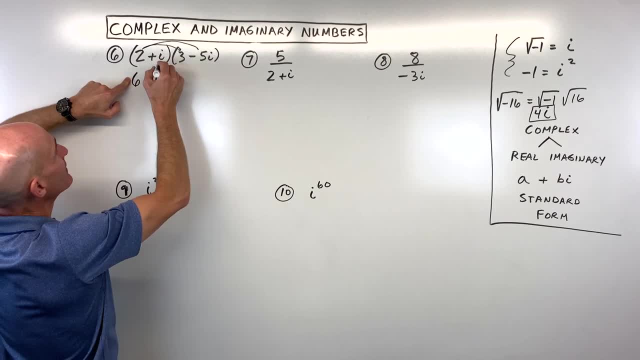 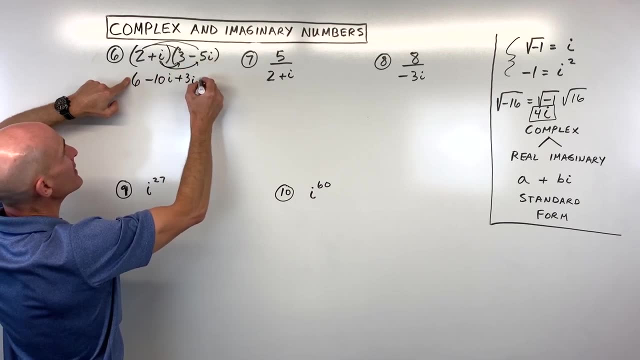 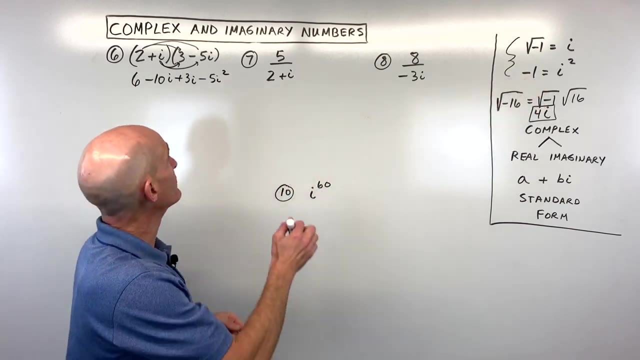 Two times negative five: i is negative ten i. Then I'm going to distribute the i. So i times three is three i And i times negative five: i is negative five, i squared. Now we know over here: i squared is equal to negative one, So we have a negative one. i squared is a negative one. 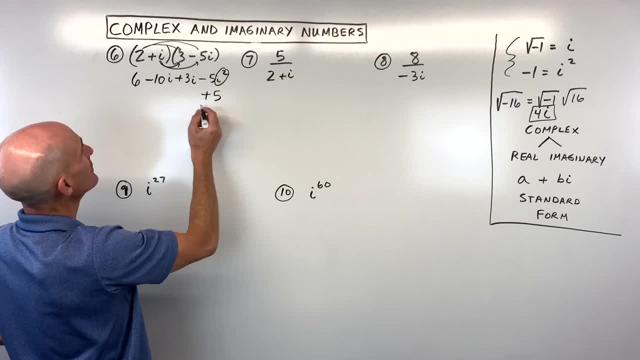 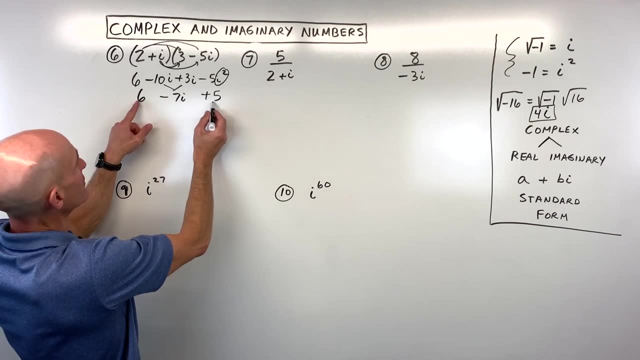 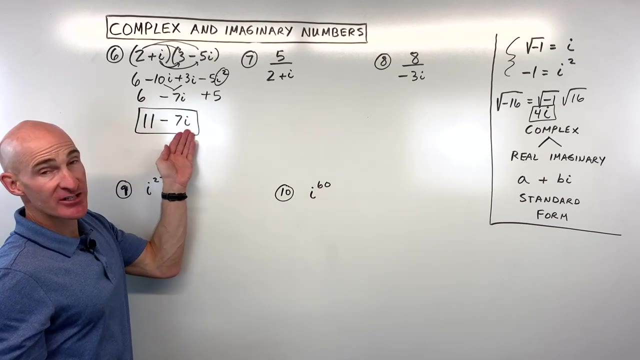 times negative five is positive five. Here we have negative ten. i plus three. i is negative seven. i Bring down the six And again, combining like terms: six plus five is eleven minus seven i. And we have it in that standard form with the real number first and the imaginary number second. 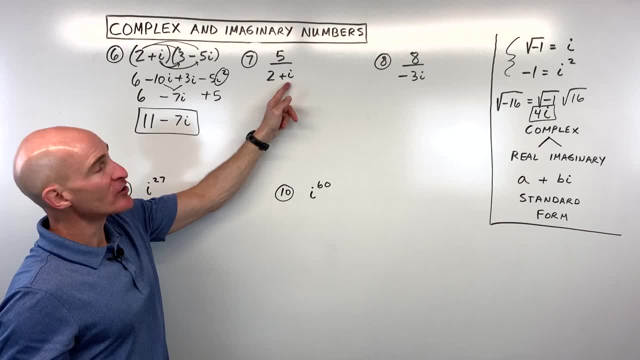 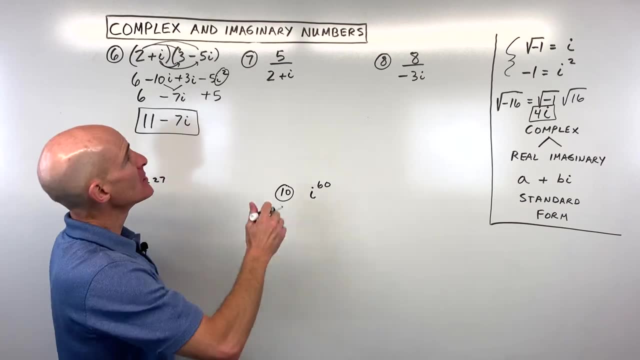 Okay for number seven. now we're dividing, And when you're dividing you don't want to have i in the denominator. That's considered improper, Just like you don't want to have a radical or a square root in the denominator. So what we do when it's a binomial, like two terms, like this: 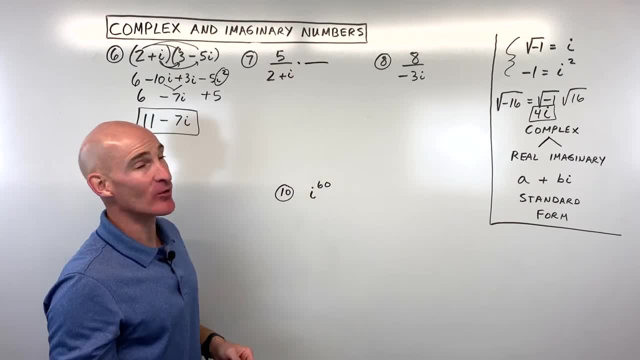 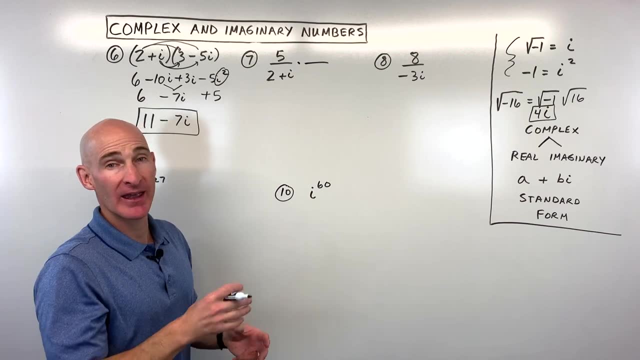 we multiply by the complex conjugate. What's the complex conjugate? If you have a plus b i, you multiply by a minus b i. Or if you have a minus b i, you multiply by a plus b i. So you just change that sign in between. So here we're going to multiply by 2 minus i. 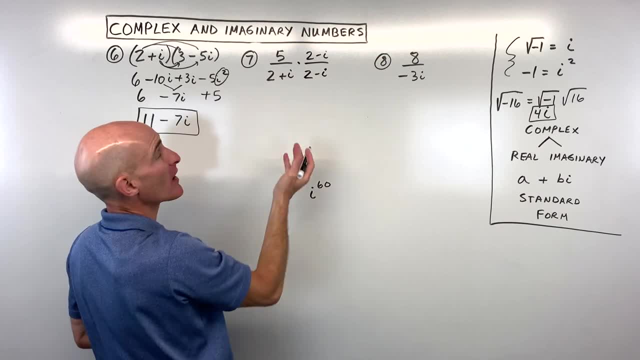 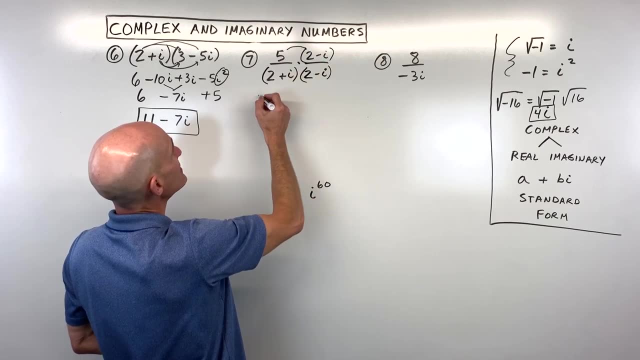 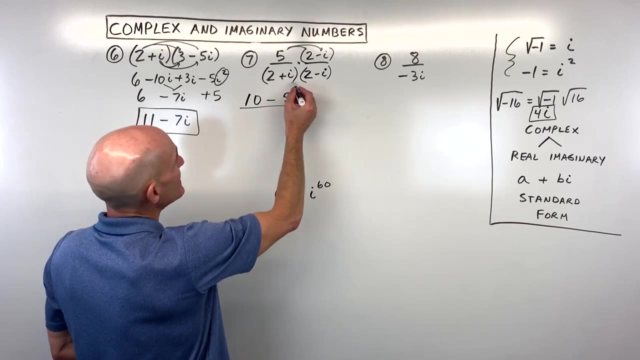 Whatever you do to the denominator, you want to do to the numerator, because that's like multiplying by one, And now what we're going to do is we're going to multiply these together. So 5 times 2 is 10.. 5 times negative i is negative, 5 i In the denominator. what's interesting is the inside and 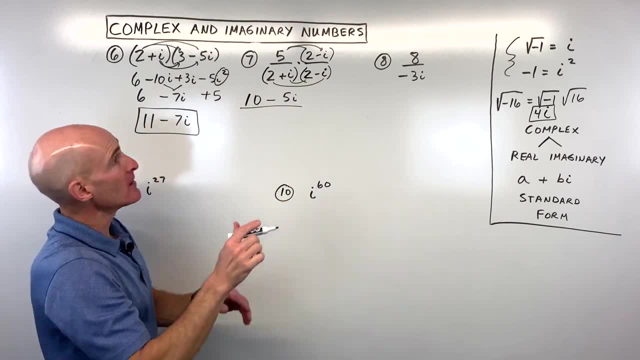 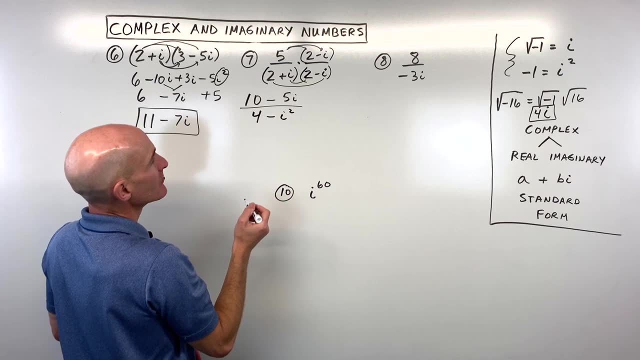 cancel. We have 2 i and negative 2 i. That's 0.. So we just get 2 times 2, which is 4.. i times negative i is negative i squared. i squared is negative 1 times this negative is a positive 1. So that: 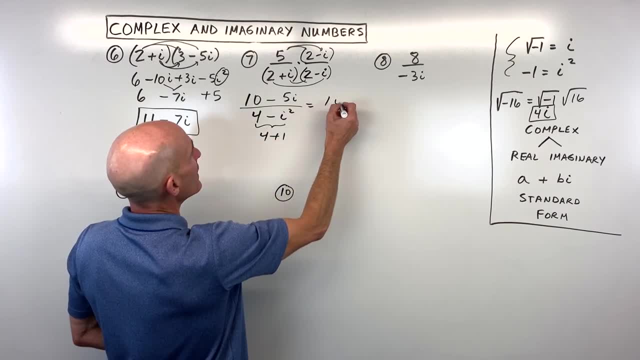 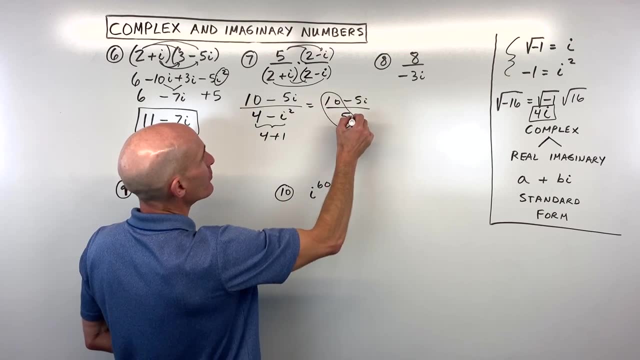 becomes 4 plus 1, which is 5.. So we have 10 minus 5, i over 5.. And you don't want to leave it like that. You want to split this up into two parts: The real part and the imaginary part. 10 divided. 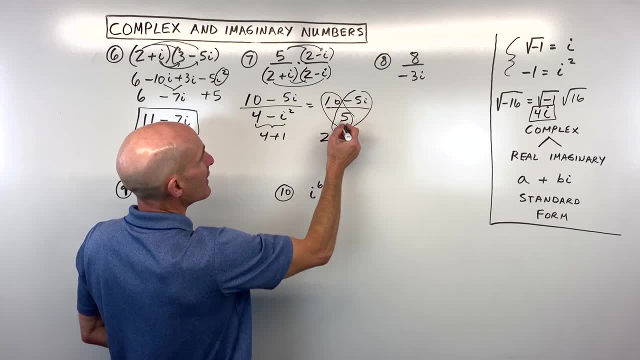 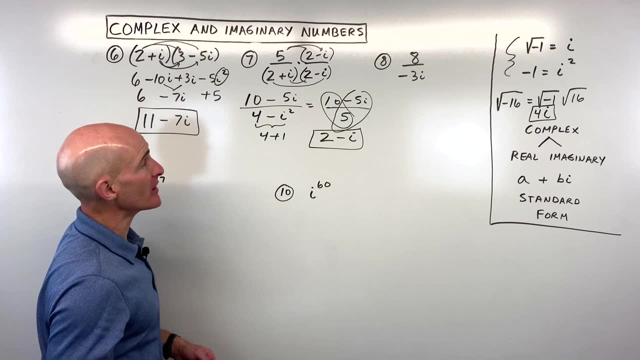 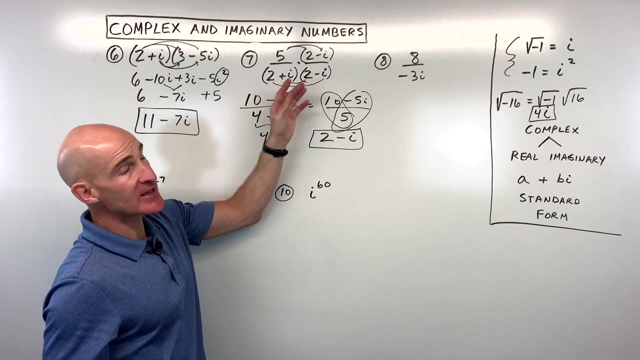 is 2 and negative 5 divided by 5 is negative 1 i Okay, so you've got it in the standard form: real plus imaginary. Now here I did a little bit of a shortcut, where I did the inside and outside cancel and then I just did the first multiply together in the last. If you don't like that method, just 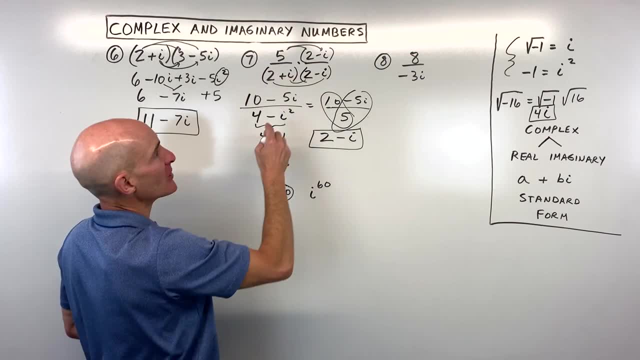 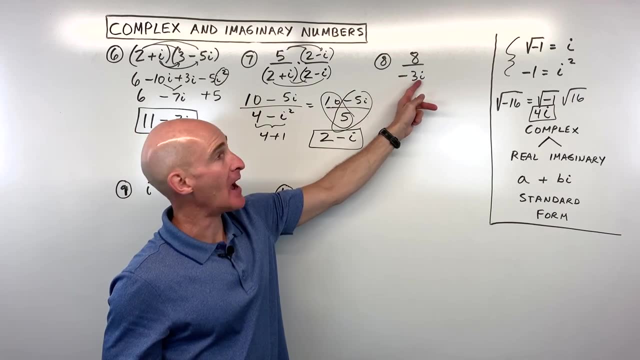 distribute twice. Distribute the 2, then distribute the i and you'll see the cancellation that occurs. Okay, for number eight. now we have a monomial or just one term in the denominator, But we still have that i in the bottom, which is considered improper. So how do we get rid of this? 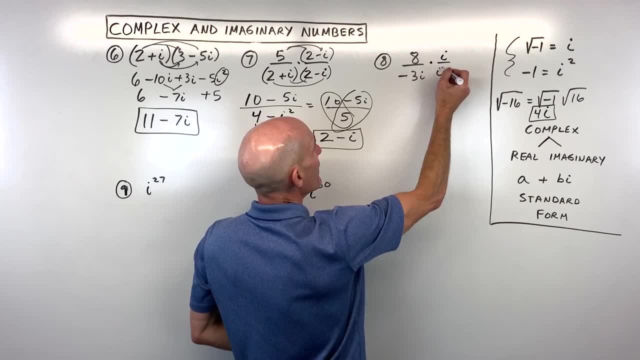 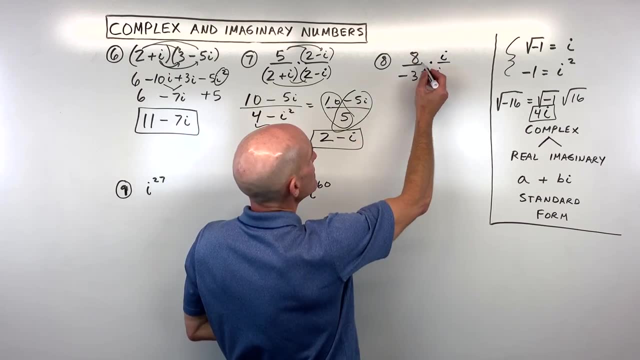 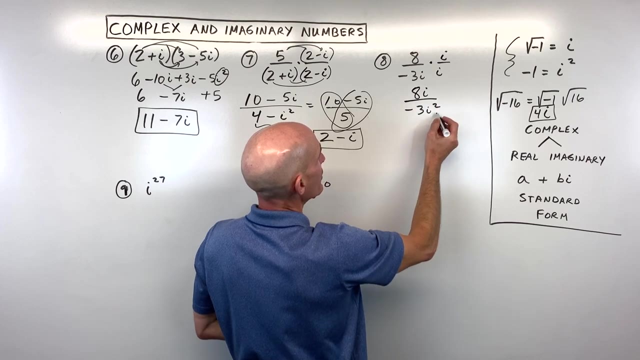 i. Well, here we can just multiply the numerator and denominator by i. i over i is equal to 1.. 1 times. anything is not going to change the value, It's just going to change the way that it looks. So 8 times i is 8i Negative. 3i times i is negative, 3i squared. 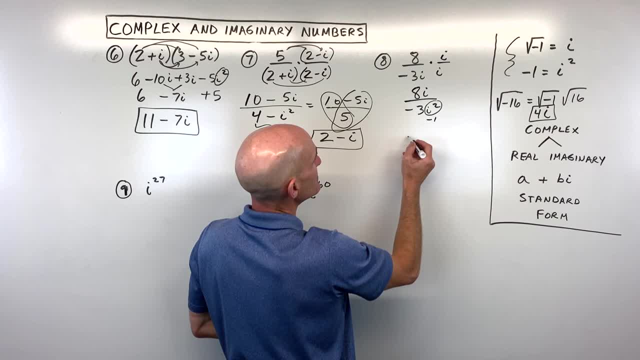 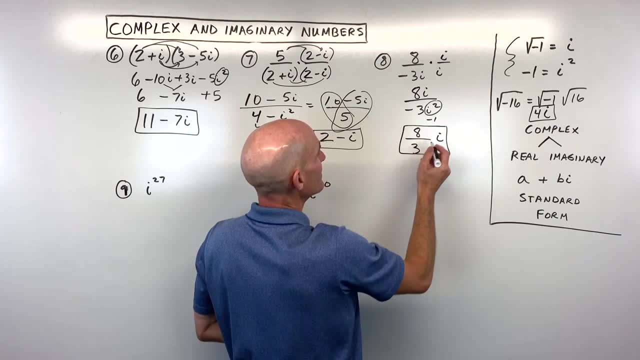 i squared. we know is negative: 1. A negative 3 times a negative, 1 is a positive, 3. We get 8 thirds. i Okay, good. and then for number 9 and number 10. this is what I call. i to a higher. 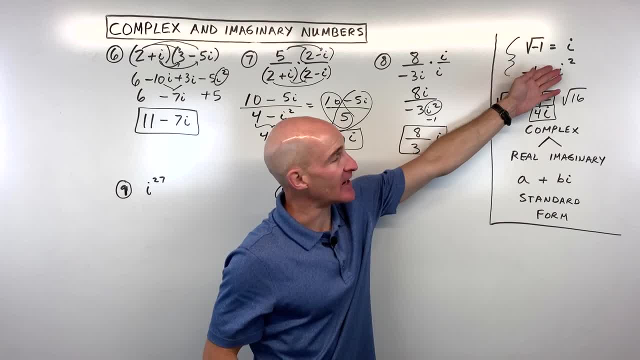 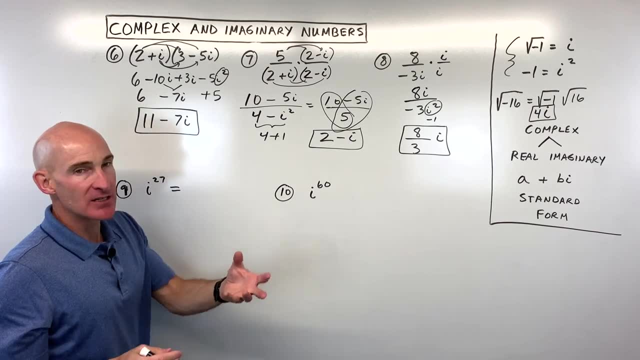 power. Like you know, instead of just i to the first or i to the second, it's like i to a higher exponent And you can see i to the 27th. the way I like to do these problems is I like to divide out groups of two. So what I mean by that is you could write this as i squared: 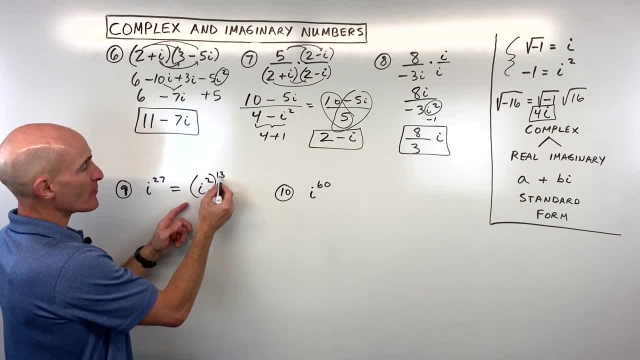 to the 13th power. See, because power to power, you multiply 2 times 13.. It's 26.. We need one more, i. So let's multiply it by i to the first. Now, the reason I do that is because i squared is negative 1.. Right and negative 1 is easy to. 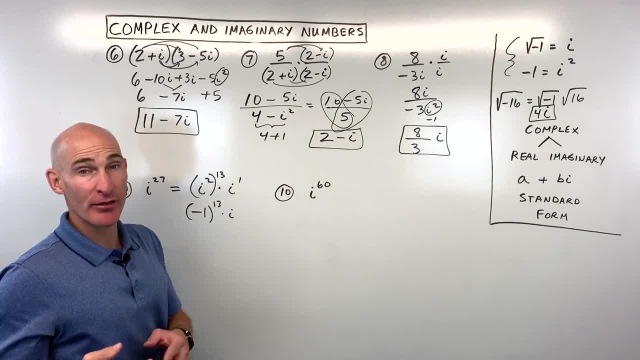 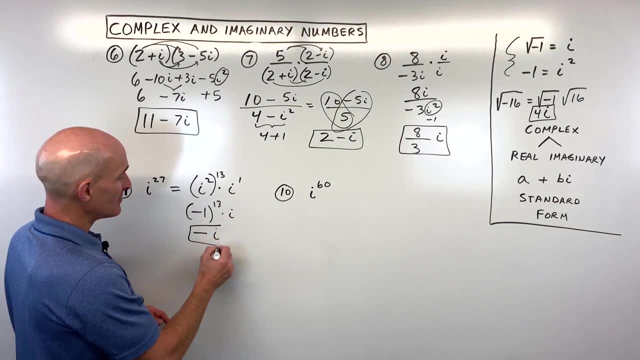 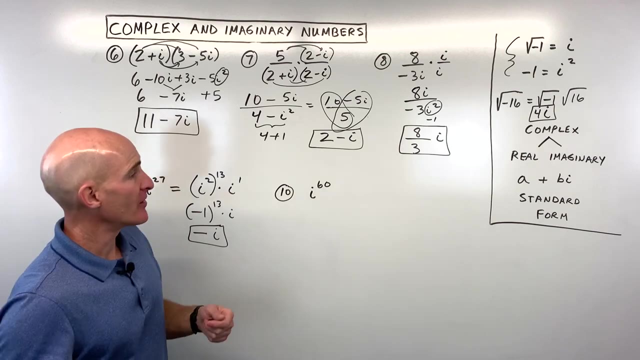 work with A negative, 1 times a negative, 1 times a negative 1.. Like, 13 times a negative to an odd power is going to be negative And then times this i is just going to be negative i. So it's an easy way to simplify. Some teachers explain it where it repeats, Like here I'll show you i to the 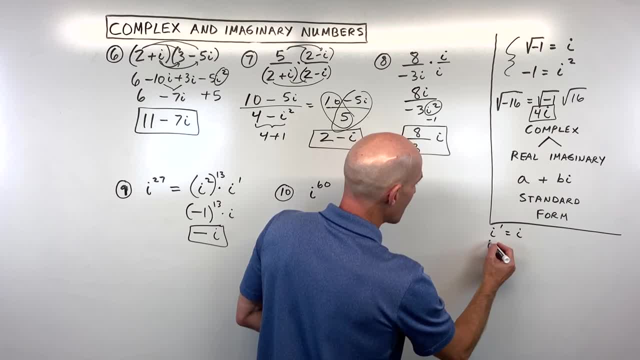 first They say: is i and then i squared is negative 1.. And i to the third is negative: i and then i to the fourth is equal to 1.. And then it repeats: i to the fifth, sixth, seventh, eighth, nine, ten, eleven. 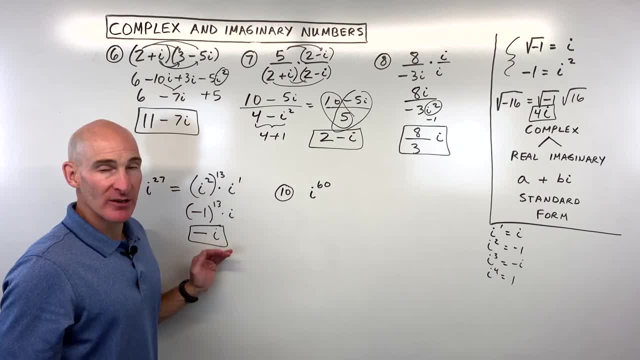 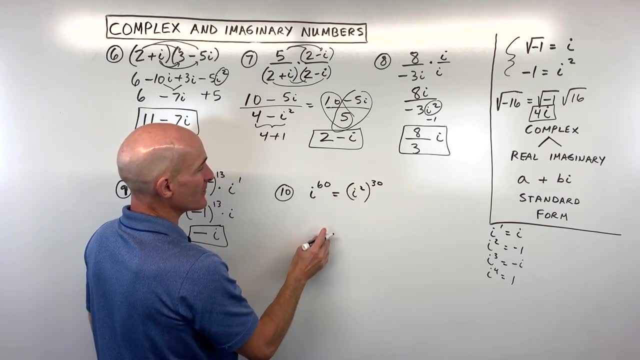 twelve. I find this to be a little bit easier, a little bit less to memorize. So for i to the 60th. let's do the same thing here. Let's see, 2 goes into 60, 30 times. See, power to power, you multiply. 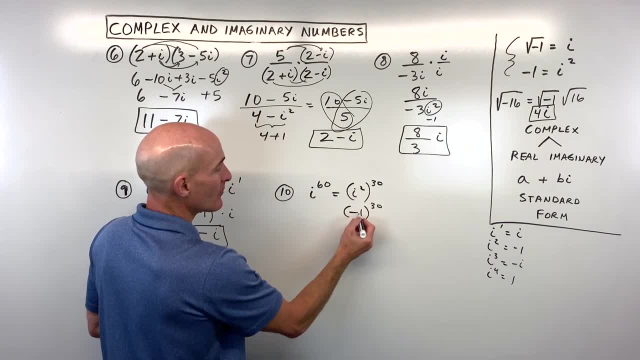 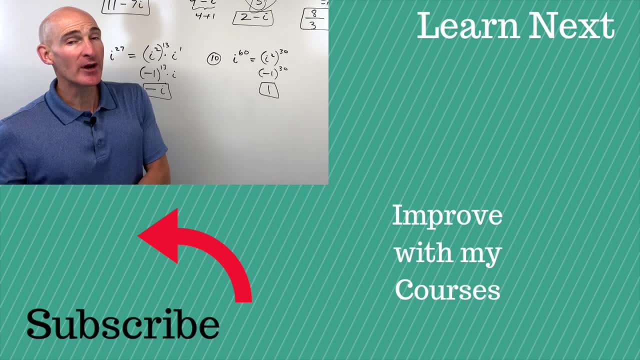 We know i squared is negative 1.. A negative number to an even power is going to be positive, So this just comes out to positive 1 and you simplified it So great job if you're able to follow these examples. If you want more, 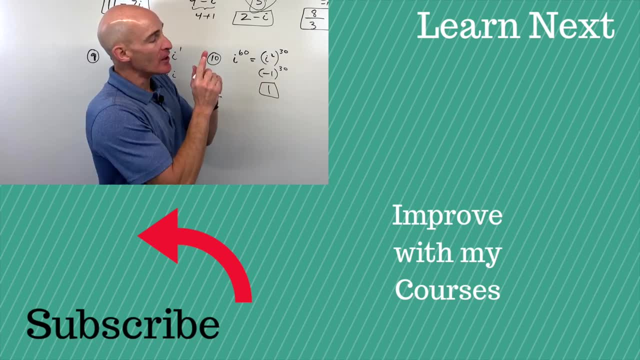 practice and you want to test yourself, follow me over to another video I did on the same topic: adding, subtracting, multiplying and dividing complex and imaginary numbers. Check out that video and I'll see you over there.